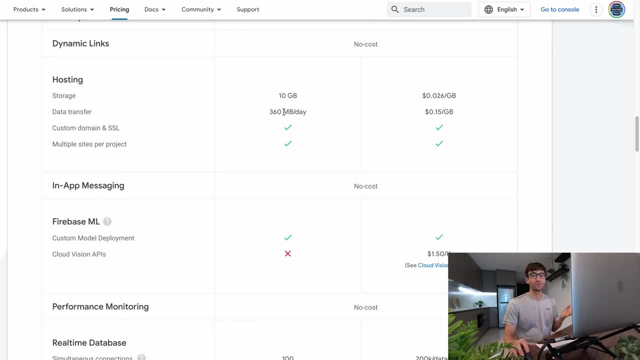 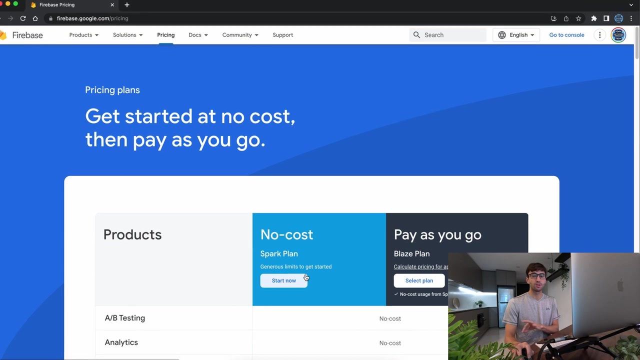 website to just get started with web hosting on Firebase, You get a custom domain and SSL for free, and you can have multiple sites per project. So that's great. We're going to start by configuring our project within the user interface and then we're going to finish up on the command line, because that's where the power. 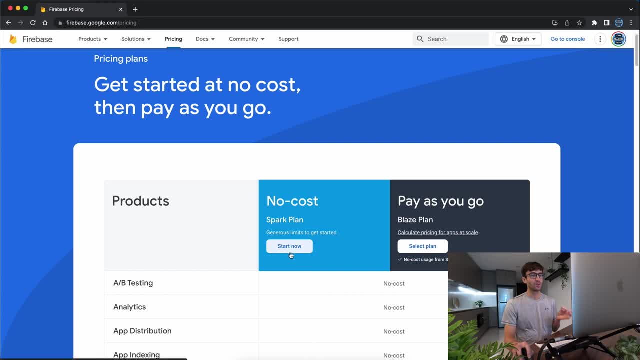 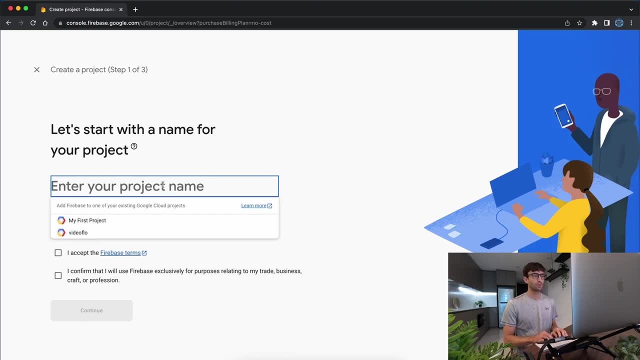 of Firebase really comes through on the command line. So let's start that and create our project in here. So we'll click create a project and the project name for me is going to be called. let's just call it Fire Tony. Okay, so we'll accept the terms and conditions for both of these. 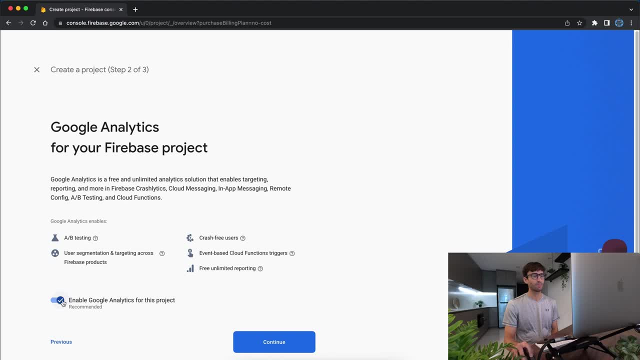 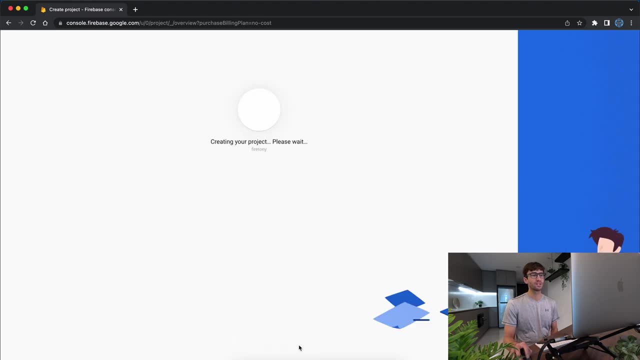 and click continue, and I'm not going to enable Google Analytics for this project. You can if you want to, but I'll go ahead and create the project and let that do its thing. All right, at this point your project is ready, so we'll go ahead and click on continue, which takes you to. 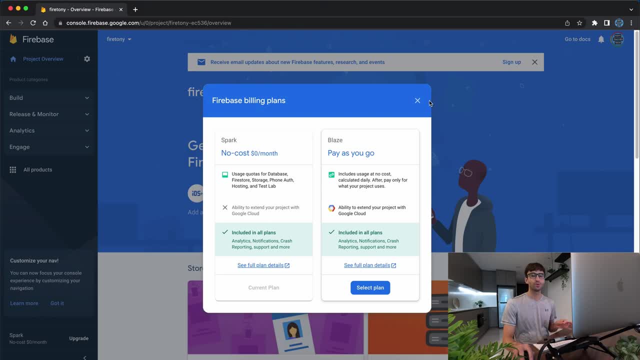 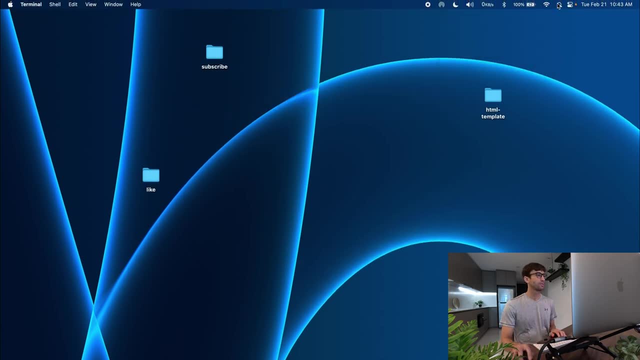 your Firebase console dashboard, and at this point we're going to switch over to the command line, So let's minimize this, and if you're on a Mac, you can open up a terminal window. If you're on Windows, you can open up a command prompt, and what you're going to need in either case is something called. 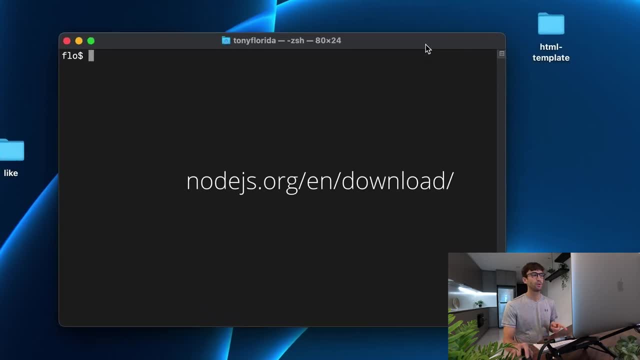 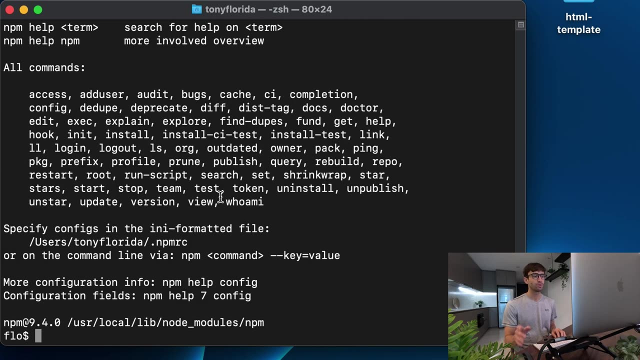 node package manager or npm. So I'll have a link on the screen here you can download and install that from nodejsorg. I already have that command installed, as you can see here. So once you do have it installed, we can get Firebase tools. We can install Firebase tools on our system with npm. 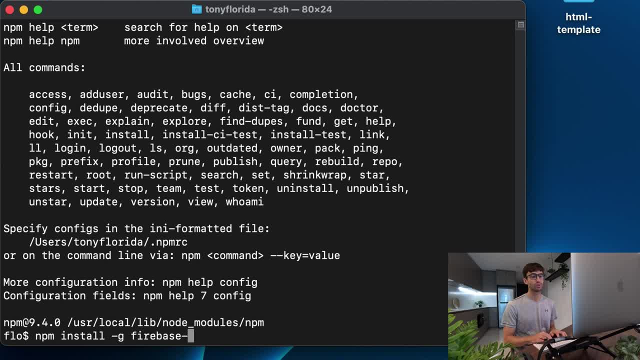 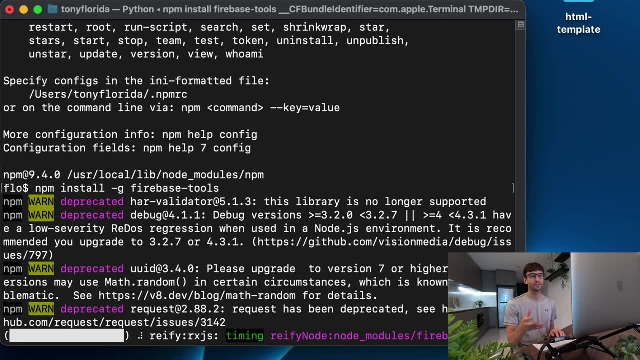 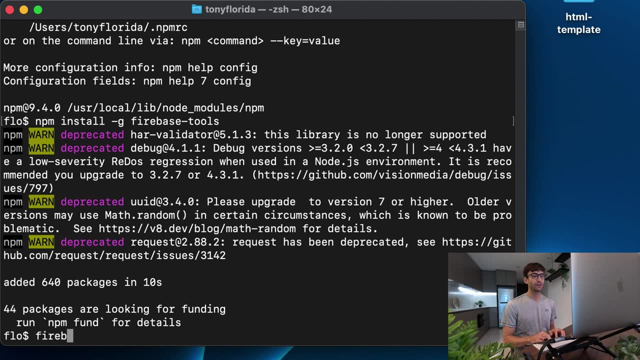 install dash g, fire base, dash tools. So execute that. That'll go ahead and download those packages onto your system and we'll let that do its thing and catch up with you when it finishes. Okay, and that finished up pretty quickly, so now we're going to use the Firebase command to log into our Google account. 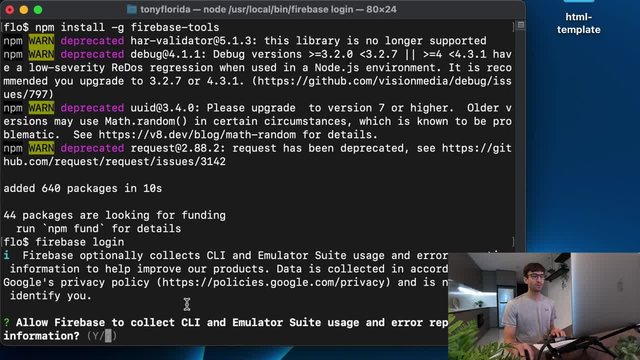 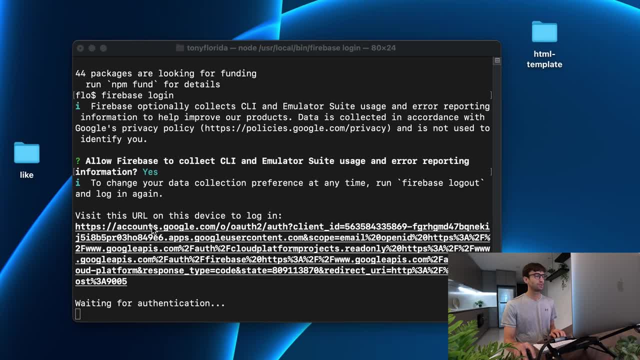 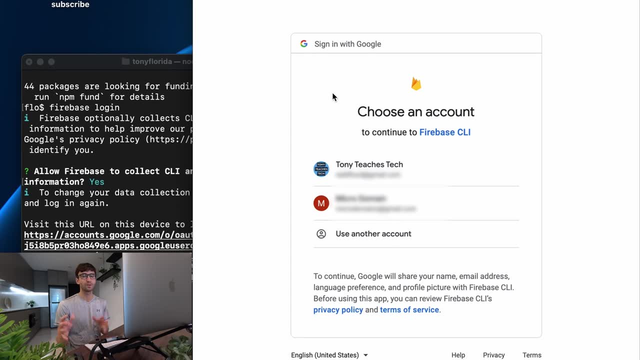 with Firebase login. So execute that and what that's going to ask. do you care if it collects usage and error reporting information? So you can choose yes or no. and what that's going to do on my website. So if I go to my website window, it opens up a tab where I can log in to whatever account I 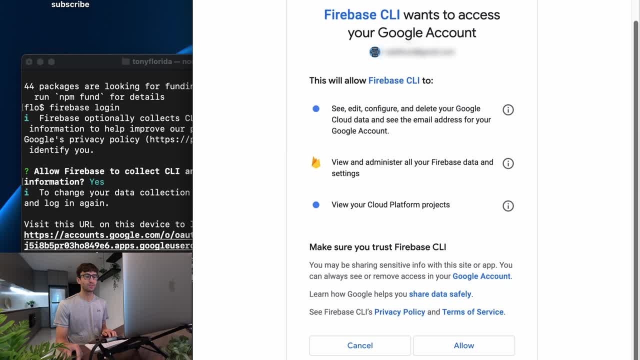 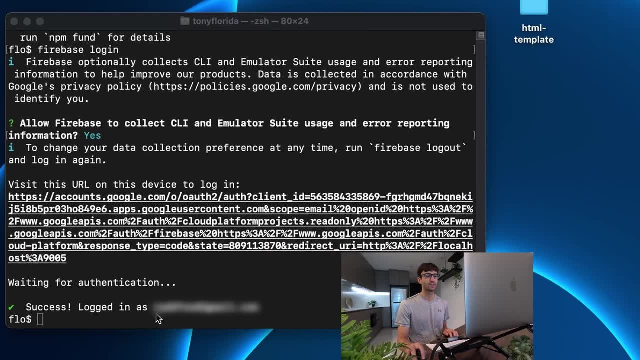 want to associate this Firebase with. So I'm going to pick this account right here and then scroll down, click on allow and it says you're logged into the Firebase command line interface. So we can close out of here and back here. we see success logged in as my email. All right at this point. 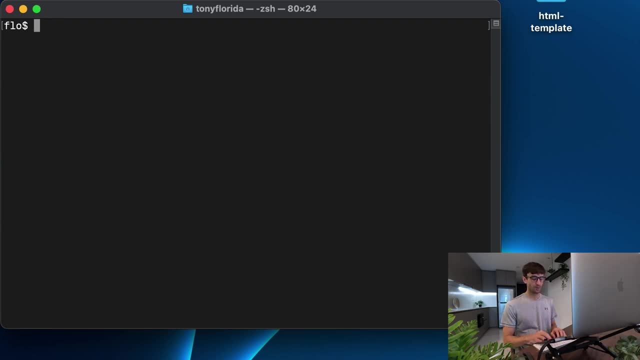 with all that setup out of the way, we can actually start hosting a website. So I'm going to go to my desktop. Okay, I'm going to choose to host my website out of. you can pick any directory on your system that makes sense and what we're going to do to start that is type in firebase init hosting. 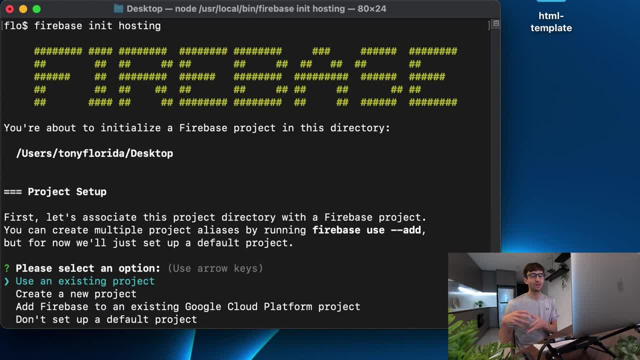 So this is going to ask you basically to associate with a project, which we only have one project at this point, So you can create a new project, but I'm going to use an existing project, just using my arrow keys and the enter key to move around here. And there is the. 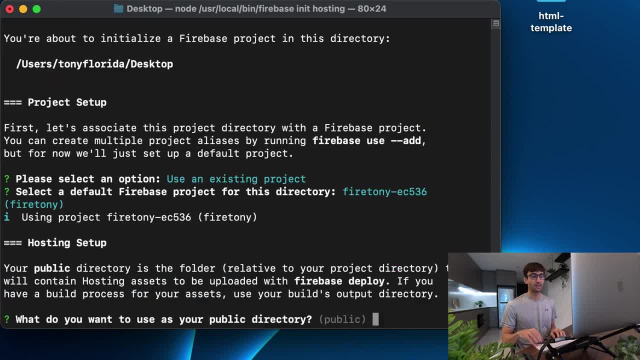 fire Tony project. so we'll associate our hosting with that. And now, where do you want your project to live on your local machine? I went to my desktop and it's going to create a public folder in here, or you can tell it the name of a folder that you want. I'll just say public in here and 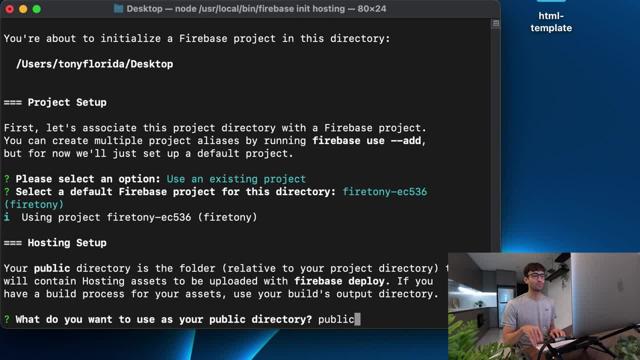 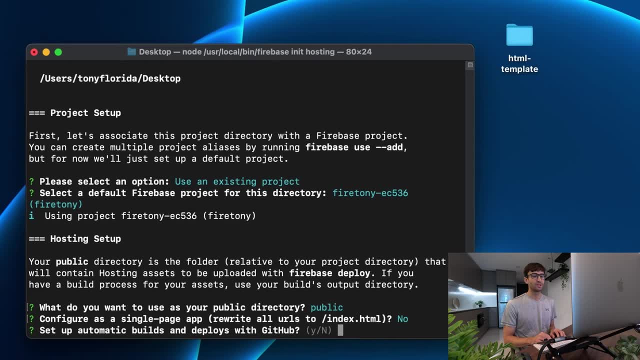 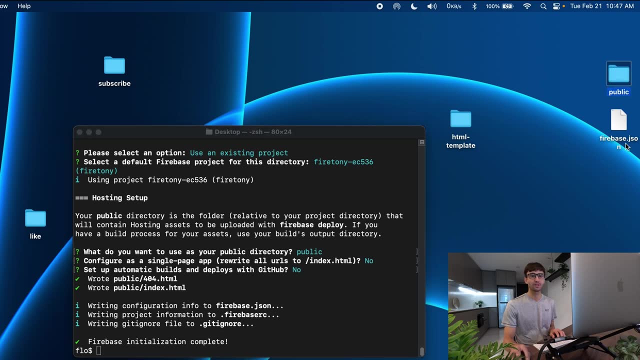 that'll still create that public directory. So let's do that: Configure as a single page app. No, Set up automatic builds and deploys. We won't do that. And now you can see when that has finished. we have this public folder that was created in this. 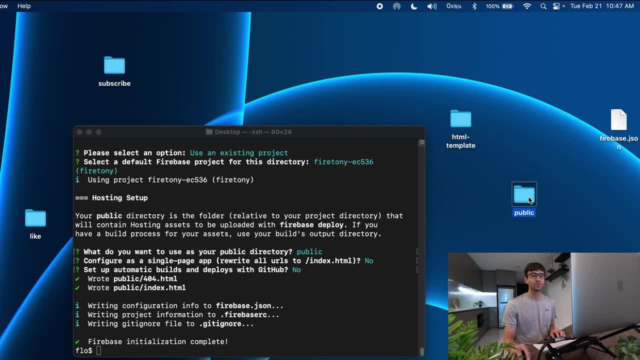 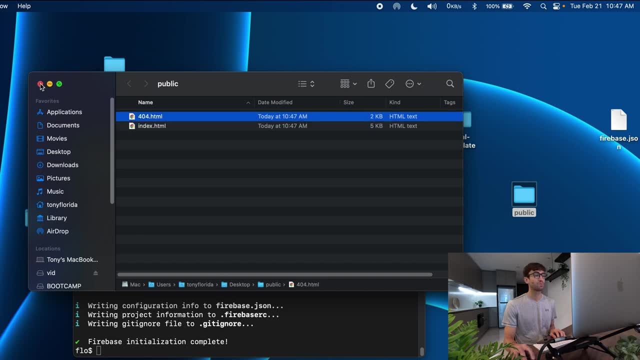 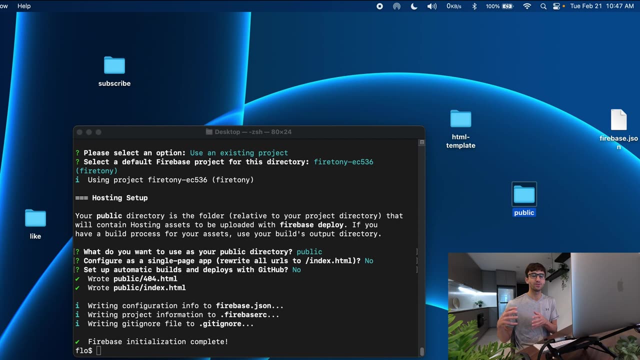 other JSON file that we won't look at too much. Let's see what's in here. Inside the public folder, we have an indexhtml file and a 404 error page- Both of them HTML files. So let's see what that looks like. How do we serve this? Well, before deploying this to a public website, let's test. 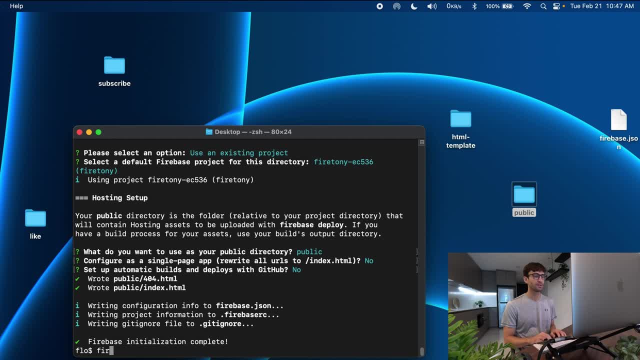 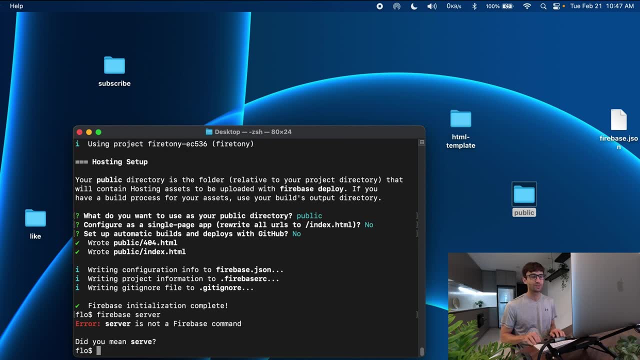 it locally And we can test it locally with firebase Serve And what that's going to do is run a local server on your computer. Whoops Serve, Not server Firebase serve. I'm sorry. What that's going to do is run a local server where. 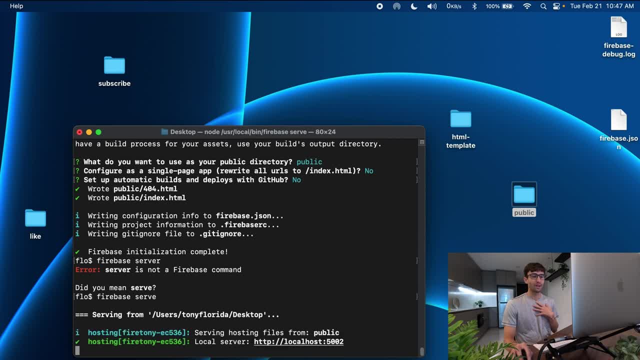 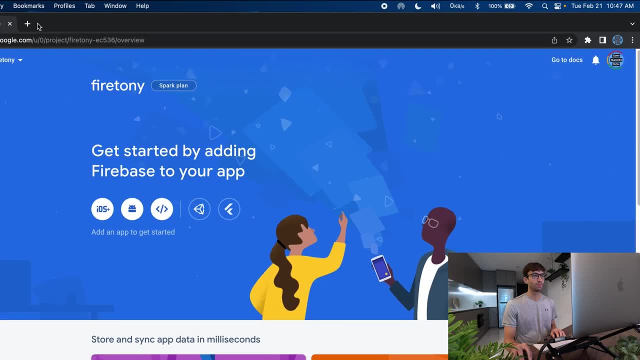 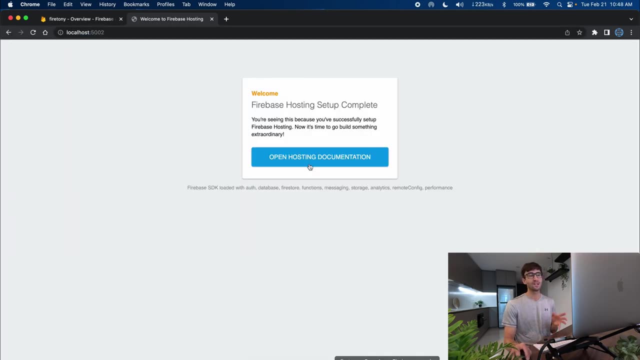 just, I can access it on my local computer And the way I can access that is at http//localhost5002.. So I'm going to open up a web browser and go to localhost//localhost5002.. And that's loading the HTML page that we saw. So let's actually prove that that's the case. Let's modify the HTML page. 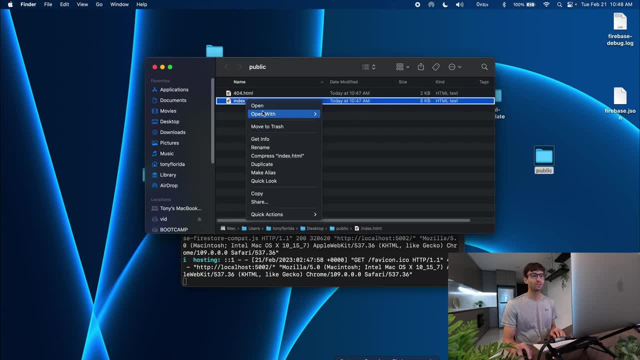 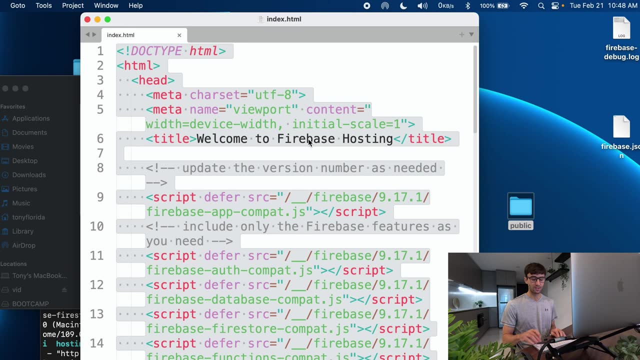 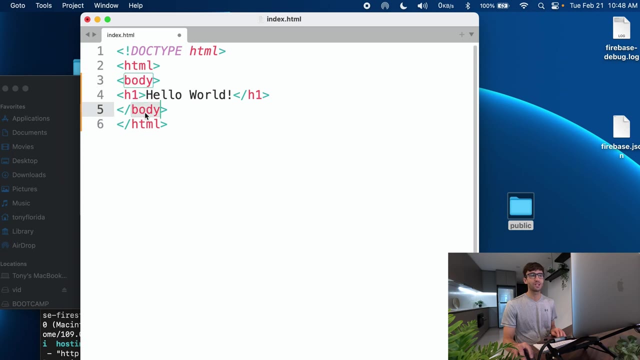 in our public directory here to say something else. So let's open that with a text editor And that does open up over here. I'm going to get rid of everything in here And I think, yep, I have some boilerplate HTML code, Some basic, just inside of my HTML body. I have one header, one element that 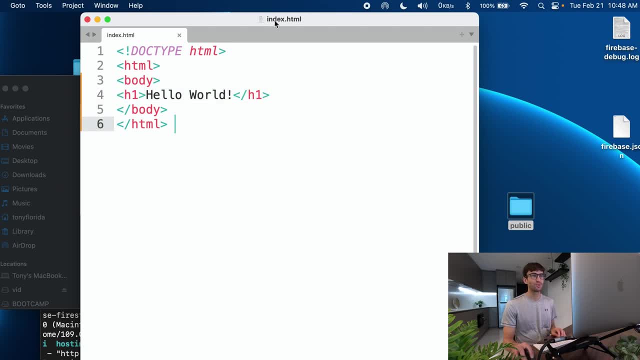 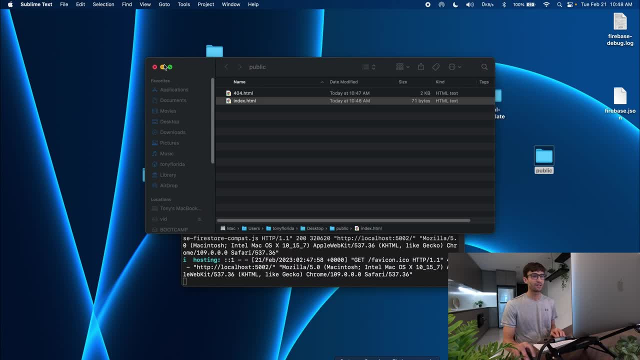 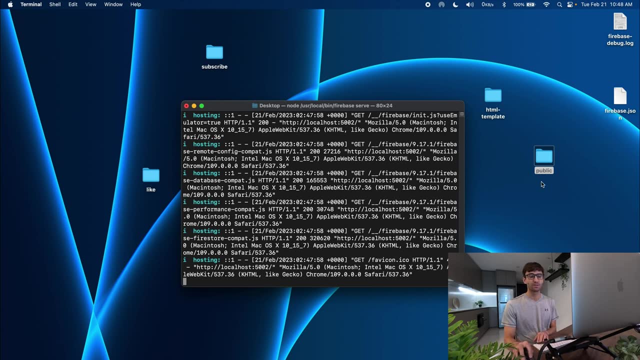 indexhtml file And I'm going to save that to the indexhtml file. I'll get out of here And we'll get out of here for now I'll. I don't even have to stop the server. It's still serving out of this. 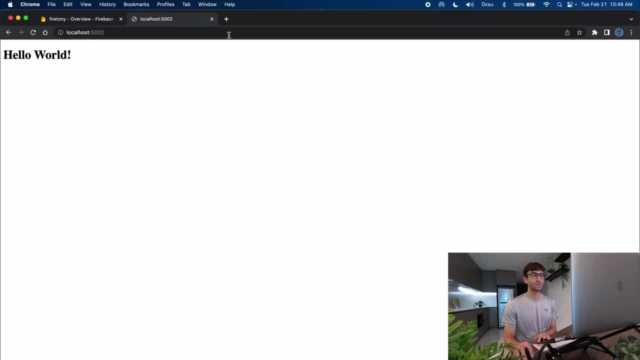 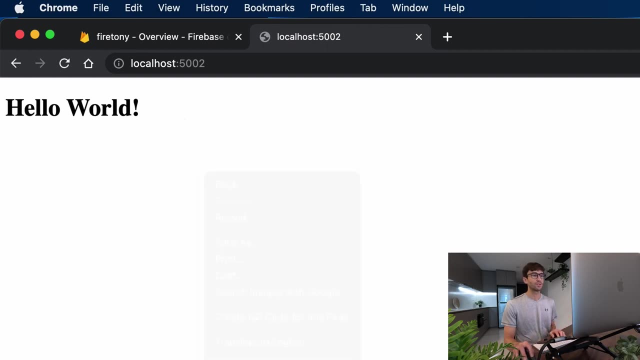 directory. We'll open up our web browser again, refresh the page And now we see our modifications, which prints out hello world as a header, one element. So if you look at the page source here, that matches up with exactly what we told it to serve, which is just those few lines of HTML. 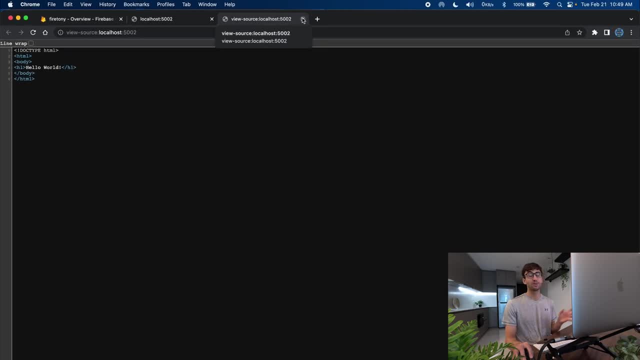 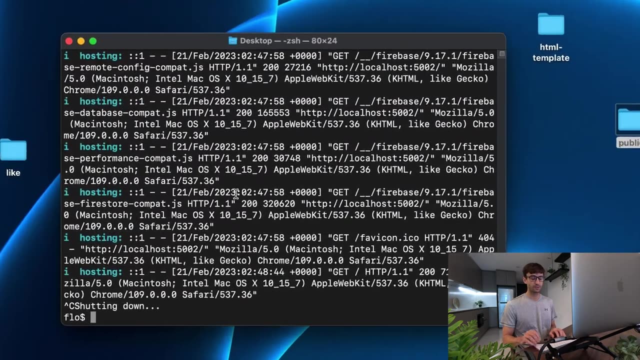 Okay, that's awesome. Let's go ahead and deploy our website to the public now. So we'll get out of here. we'll minimize this, we'll do Ctrl C to shut down our server. And now, instead of doing what we were doing before with Firebase serve, we can do. 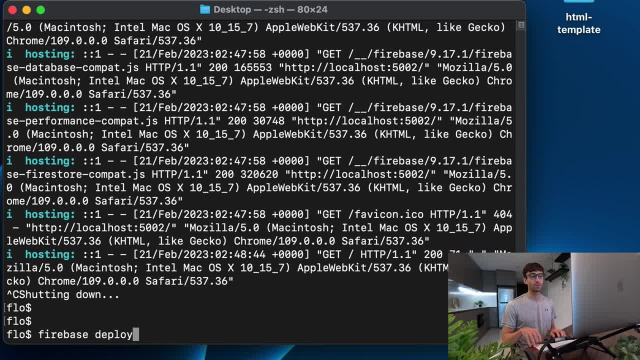 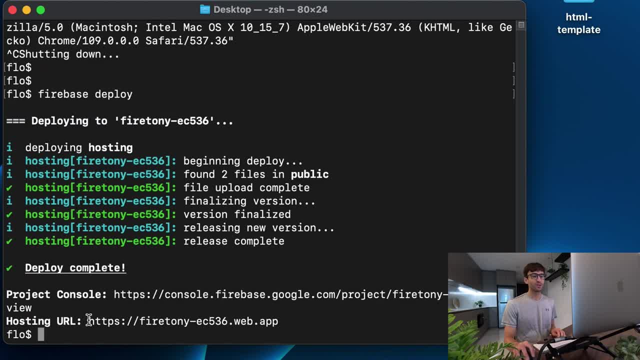 Firebase deploy and that's going to deploy it to the public, So we'll execute that And that's uploading our files to the server. And now you can see that our hosting URL is this one right here: HTTPS Firebase or firetonywebus. And that's uploading our files to the server. And now you can see that our hosting URL is this one right here: HTTPS, Firebase or firetonywebus. And now you can see that our hosting URL is this one right here: HTTPS, Firebase or firetonywebus. 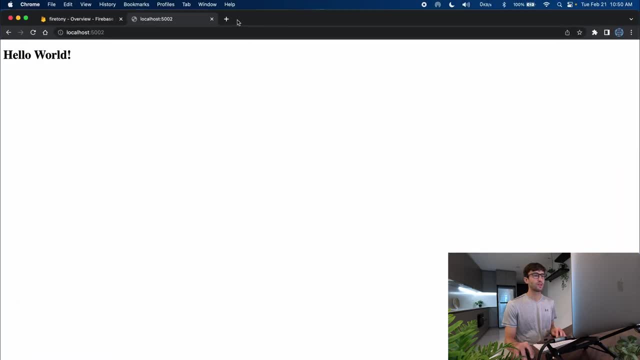 And now you can see that our hosting URL is this one right here: HTTPS, Firebase or firetonywebus. So I'm going to copy that, open a new tab, paste it in And, as expected, we see the same exact thing: US app. So I'm going to copy that, open a new tab, past it in. 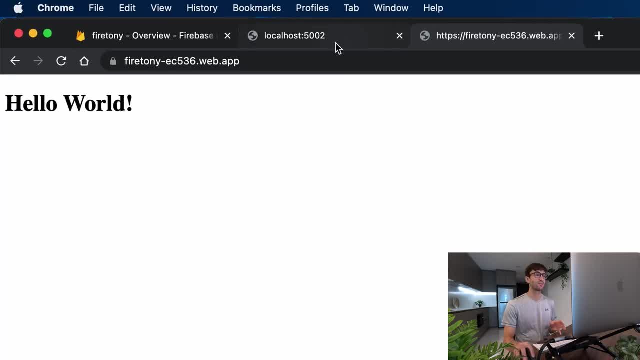 And, as expected, we see the same exact thing, But this time instead of being a local website, on our computer at localhost, but this time instead of On our computer at local host. this is publicly available. Anybody can go to this website. 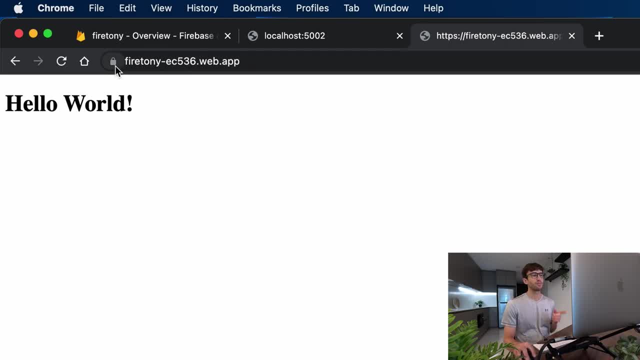 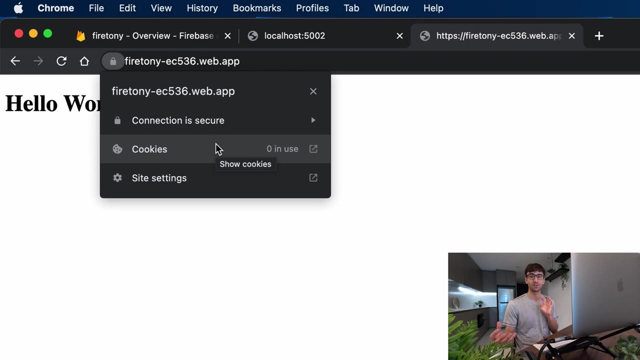 The one thing that I do want to point out here is that Firebase automatically installs an SSL certificate, so that's why you see this lock icon up here, whereas my local website does not have that. so what that means is that the connection between anybody who visits your website and your website is automatically secure, and 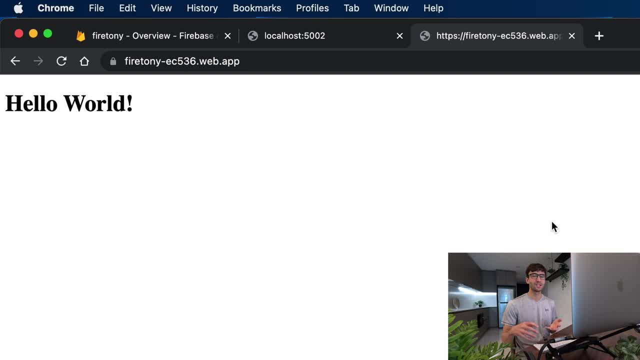 encrypted, so that's a really cool thing. a lot of other web hosts. you have to take an extra step to do that, but because we are using firebase, that comes with it for free. the next thing I want to show you how to do is to take this. 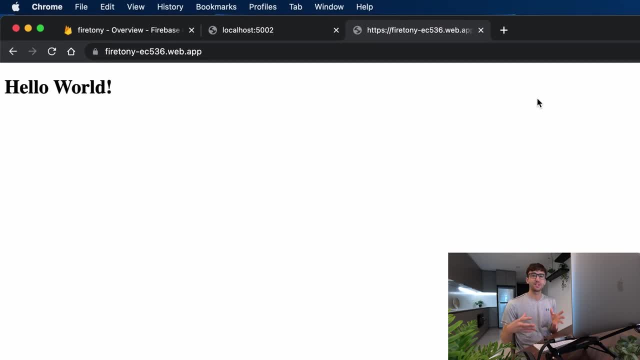 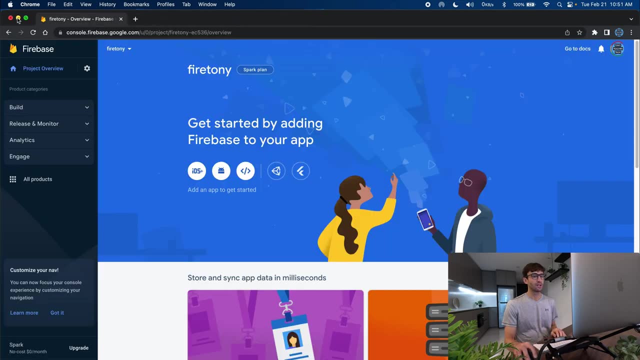 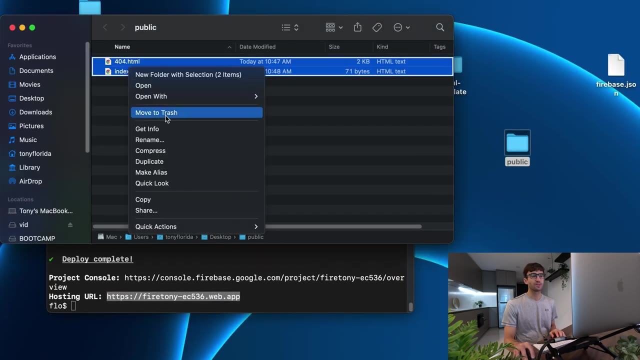 pretty drab looking website and spice it up a bit with an HTML template. so as long as it's a static website, you can do pretty much anything with it. so let's go ahead and do that in our public directory. I'm gonna get rid of everything in here, since that was just for testing purposes. I have on my 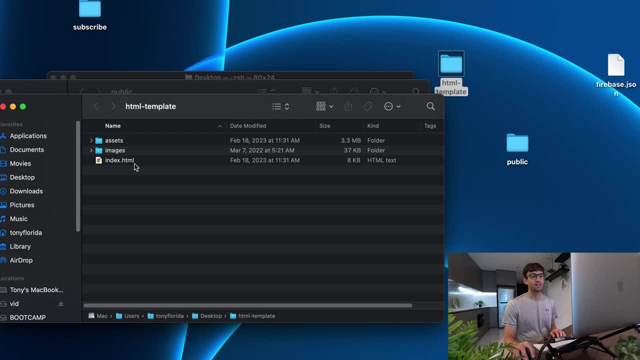 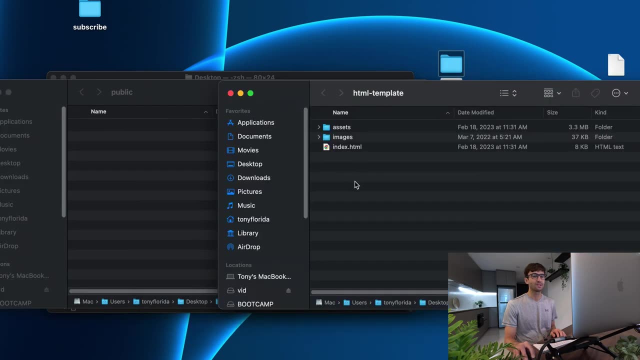 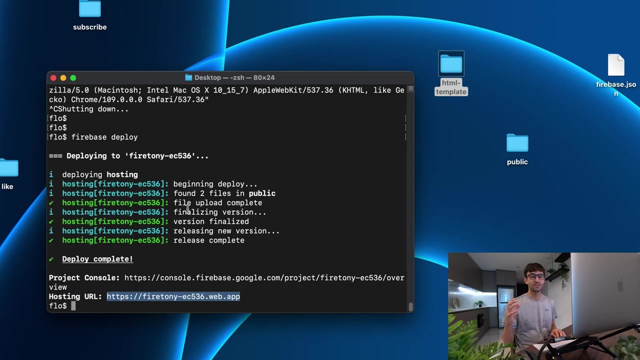 desktop, this HTML template which has an indexhtml file, some images, some assets, and that's all linked up and ready to go. so I'm gonna take contents of that and simply drag it into my public directory and close out of everything, and just as easy as we did before with the firebase deploy command. 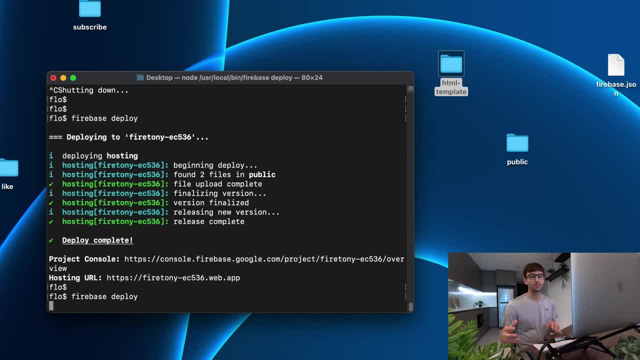 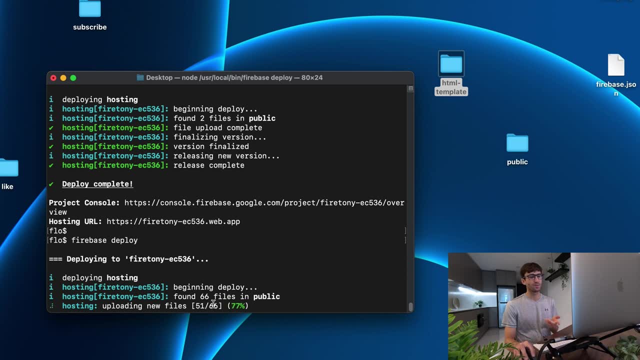 we'll execute that again. what firebase is going to do is release a new version of our website to the server, and you can see that happening here. it's uploading all those new files. this time there's 66 files, and now we can go back to the. 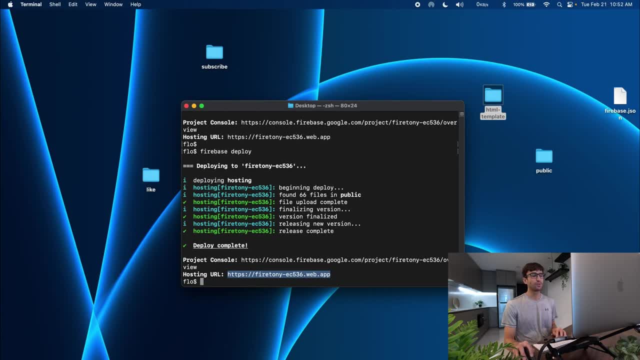 website in a web browser and see the new changes to our website, and actually you can see the changes to our website and actually you can see the changes to our website and actually you can see the changes to our website and actually, yeah, we'll do that. we'll do that. I was gonna say we can do it locally. first, to 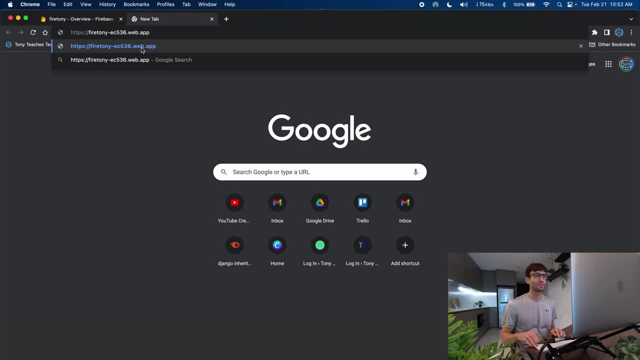 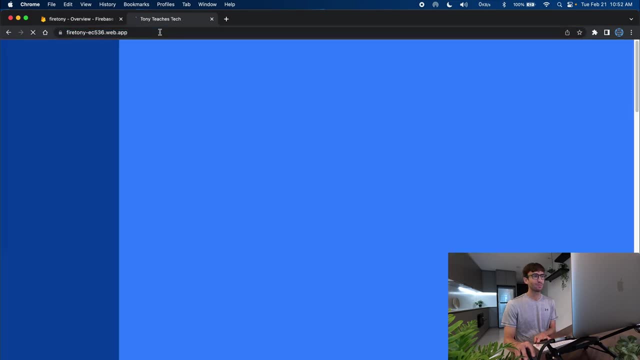 test our changes, which is a good practice, but we just went right to the public, that's okay. so we'll load that up and we don't actually see those changes happen right away. but now we refresh the page. it took a little bit, maybe some caching. now we do see those changes being applied to our website. so just a. 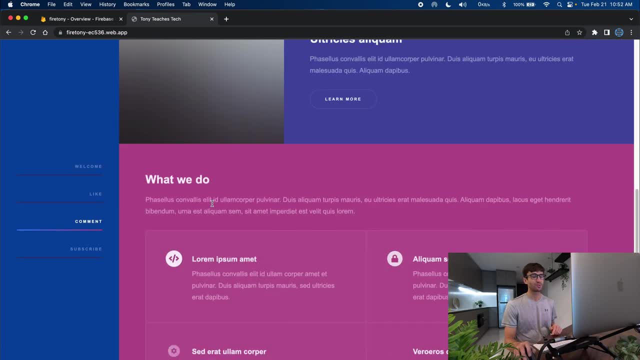 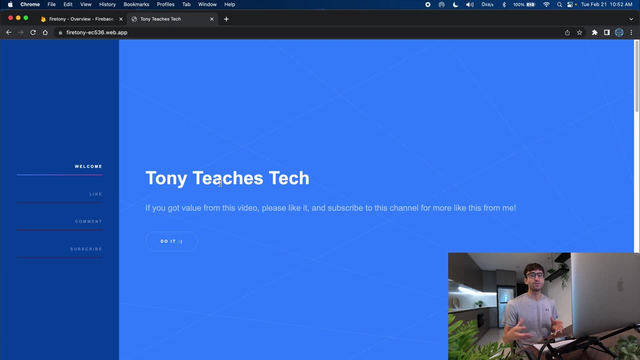 simple website with a couple links over here you can scroll down, see a whole bunch of stuff. I just grabbed this template off the internet and you can do the same thing for whatever you have in mind for this website that you're building with firebase. so in this video I also want to. 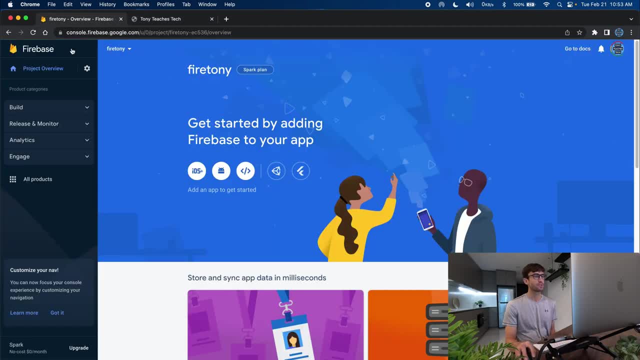 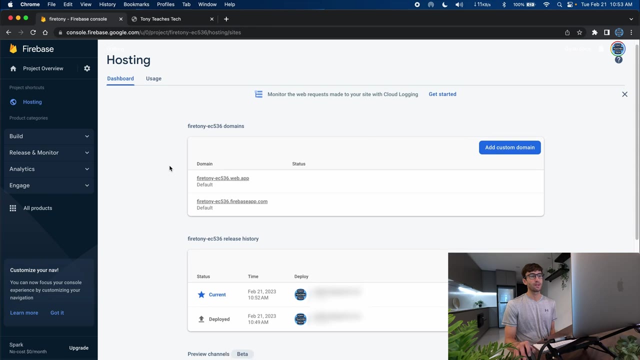 show you a quick overview of the firebase dashboard, because there's some good stuff over here. so go to your firebase console and what you can do when you expand the build menu item over here. you can go to the hosting section and kind of see what we were working on on the command line. so here is our URL. 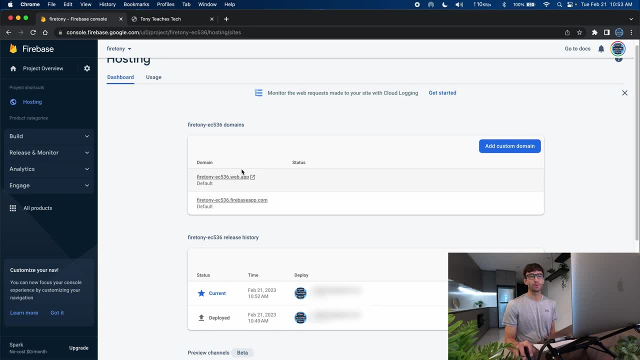 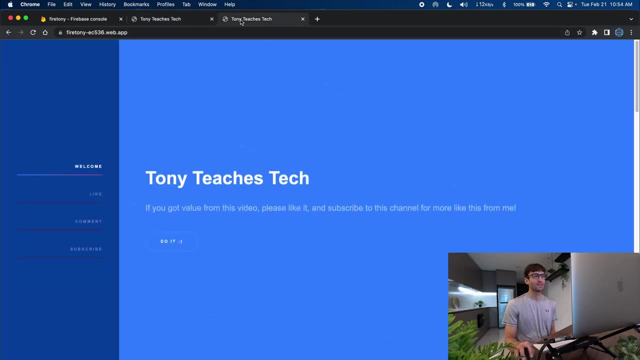 that we were accessing. there's also this other URL. they both point to the the same thing. One of them is a webapp domain and one of them is a firebasecom domain. So let's open that one, and that does indeed load the same exact website as the webapp. So think of: 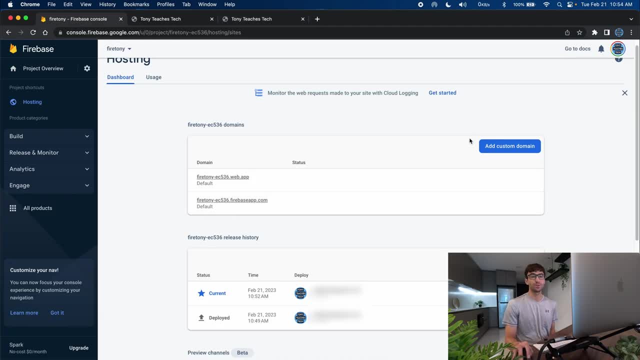 them as copies of each other. You can add a custom domain name to these so you don't have to use domain names that they provide. I'm not going to go into that in this video, but it is a pretty straightforward process. Also down here you can see all of our release history. So the initial 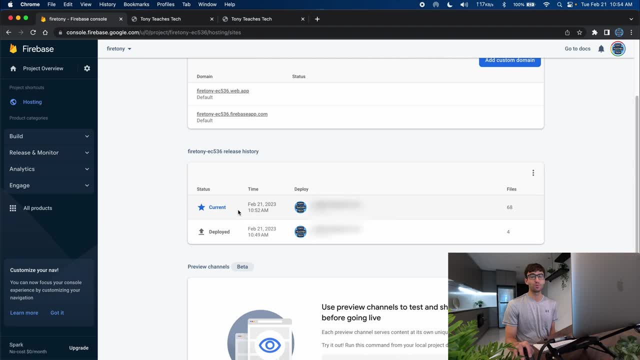 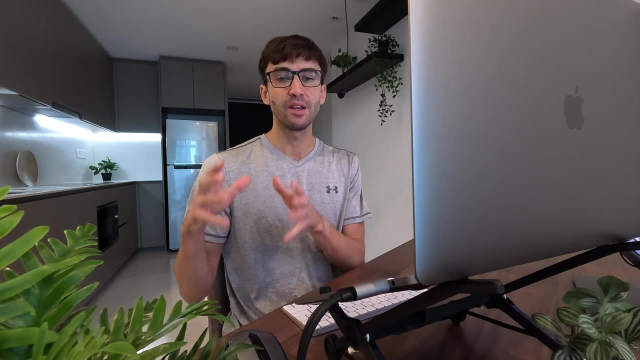 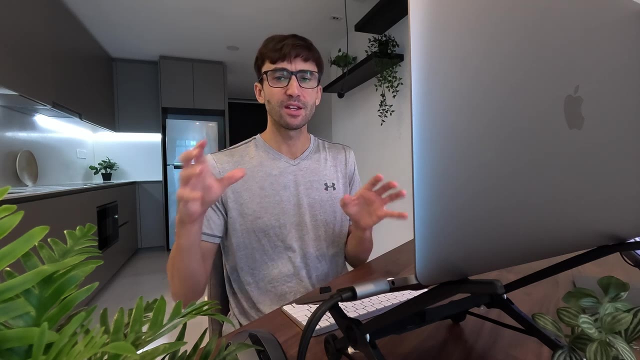 deployment that we made, and then the second one that we did with the HTML template, is right here. One last thing I want to explain to you is the relationship between Google Firebase and the Google Cloud Platform. So Google Firebase actually runs on top of the Google Cloud Platform. You can? 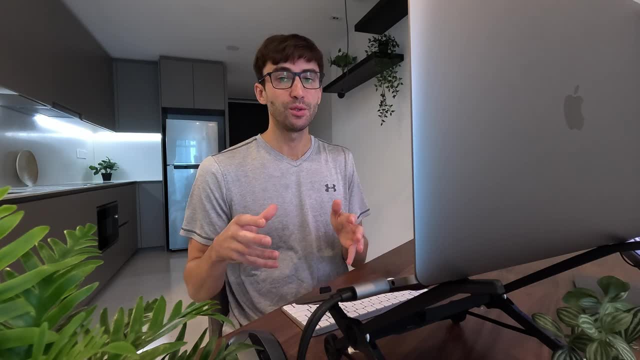 think of Firebase as a wrapper around the Google Cloud Platform, where you can actually host a website yourself, But it's a lot more technical. Firebase makes it a lot easier for people to get started with hosting on top of the the Google Cloud Platform. And just to show you that that's the case, I'm going to open. 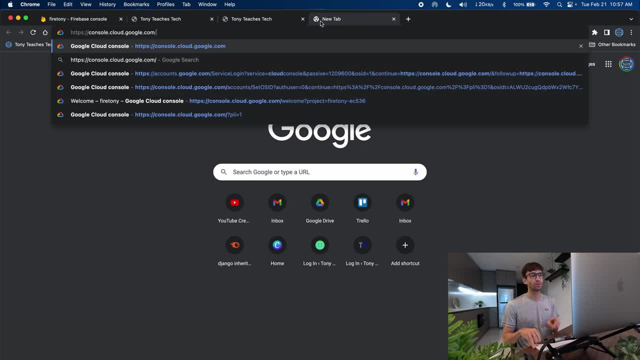 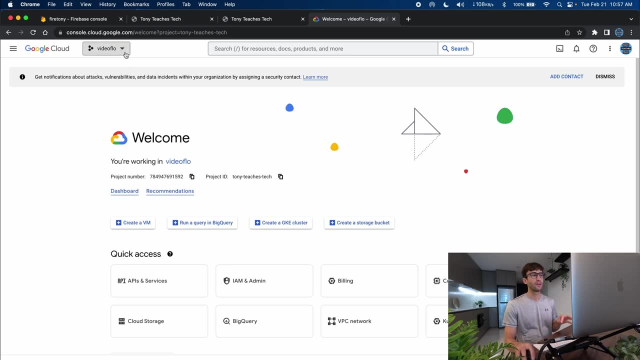 a new tab here and go to consolecloudgooglecom. You can do this too, And up here you can see your different projects. I have another project in here on Google Cloud, but you also can see your Firebase project, which is Fire Tony for me. 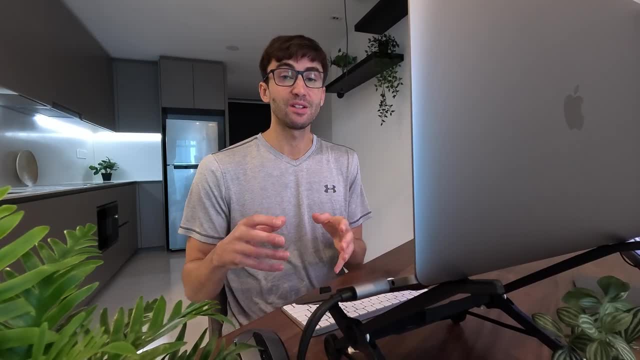 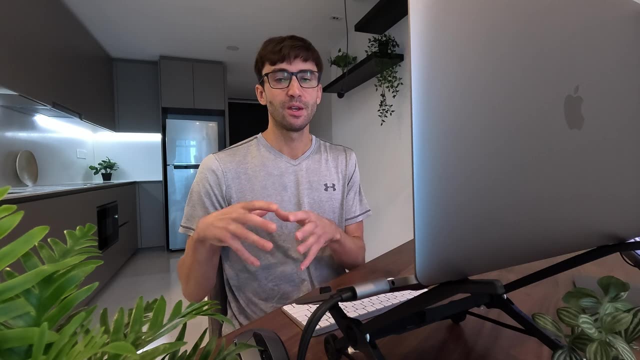 So, like I said, there is the option to host directly a website on the Google Cloud Platform. There is free tiers as well. They're less restrictive. There's more generous limitations to them, And I actually have a video about that. if you want to set up a WordPress website with a database, a dynamic website on the Google Cloud.